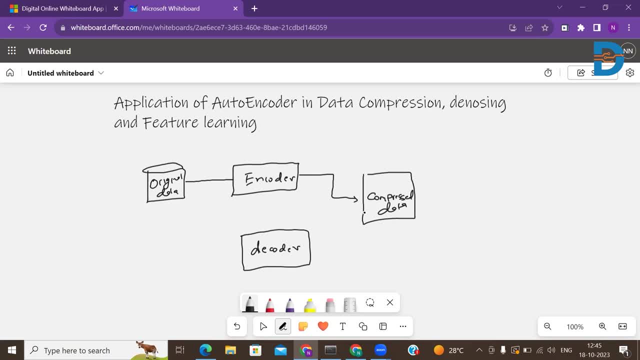 form of the compressed data. we can simply send this data back into the decoder. and what decoder will do, since it has learned all the weights, it will reconstruct my data. It will reconstruct my data. So that's what the data compression. So, of course, since the model 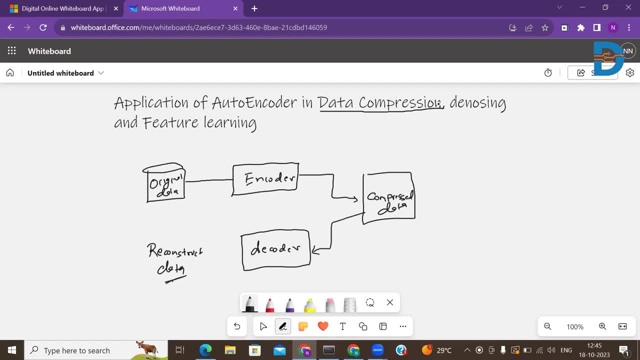 is very much optimized in terms of understanding or making the picture get back into the original state from the compressed state. we can use this autoencoder network for putting up all the data So we can put the data into the compressed form. Of course, when you have the data in the compressed 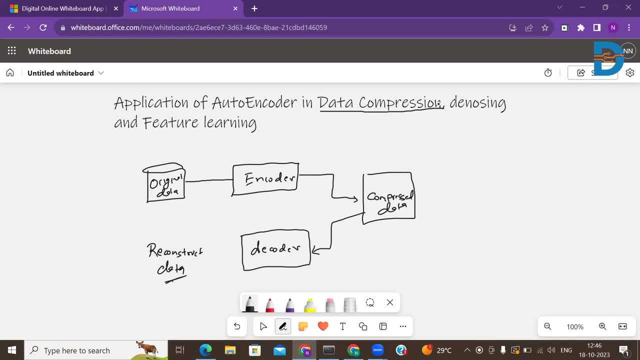 form. we can have a lot of storage right And whenever we require to have that original structure of the image back, we can simply pass the encoded one into the decoder and decoder will give me the original image of the compressed one. So that's one of the application of the 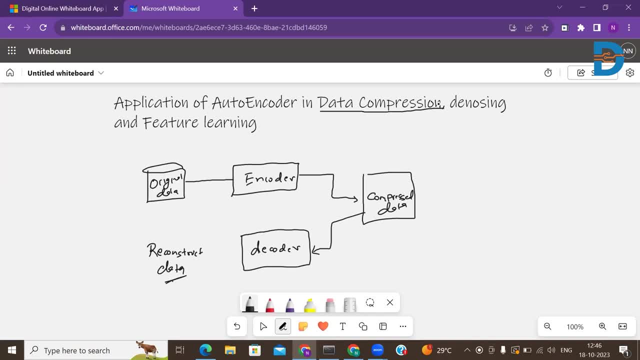 autoencoder, that is the data compression, Denoising, If you talk about denoising as such. so in the real world, raw encoder, raw encode data- is often noisy in nature. We know this, And to train a robust 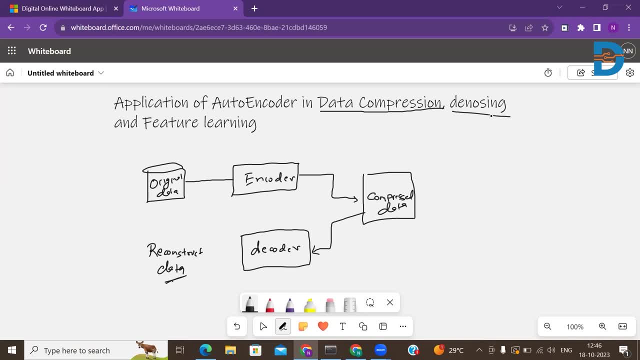 supervised model requires clean and noiseless data. So autoencoders can be used to denoise the data. So, basically, what happens that? let me just show you. So when we talk about denoising the data in this, what happens? you have some sort of image. 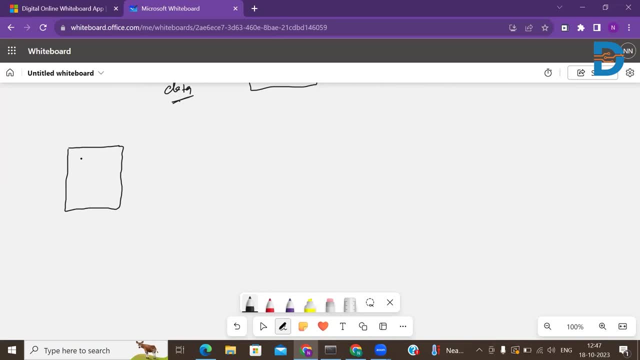 and that image is quite noisy. I mean again, you have like sample image, I'm just making it, but this image is quite noisy, right, It has lots of blurry thing And let's say, you know, the pixels are not clear. we can say: 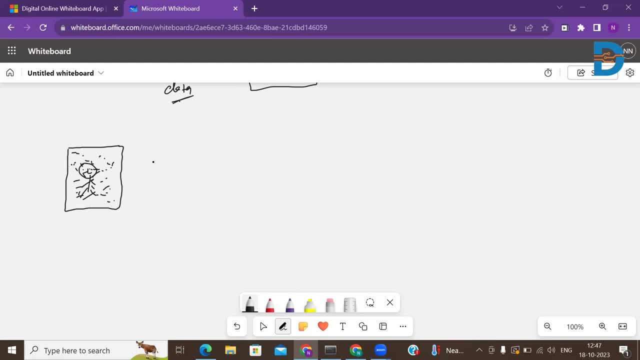 So the image denoising is, of course, one of the very popular applications where the autoencoder try to reconstruct the noiseless image from a noisy input. So what happens? that we have the input layer And that particular input layer is of course there with the hidden layer. 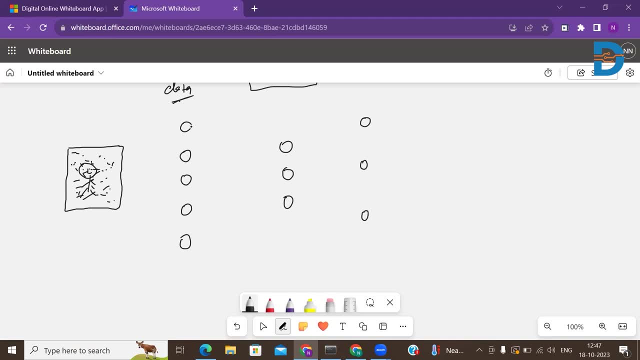 And we have the output layer like this, And you have these kind of attachments like this- You know I'm not making all the attachments, I'm just giving an example- And you have the output layer like this. So in this case, what is happening? the noisy input image is fed into the autoencoder as input. 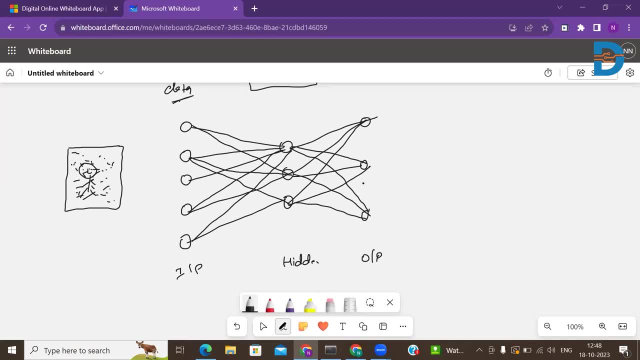 And the output is noiseless output. It is constructed by minimizing the reconstruction loss. So in the autoencoder chapter we have understood about that. what exactly the reconstruction loss, With the help of reconstruction loss itself. the machine understand that. how much you know. 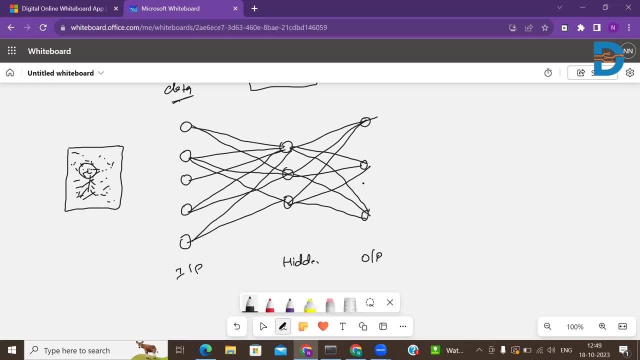 when it is making the encoded image back into the original form, it compares with the actual image and then the reconstruction loss is being calculated. So, since this model has been trained so many times and the reconstruction loss is very, very less, even if we are having a noisy input. 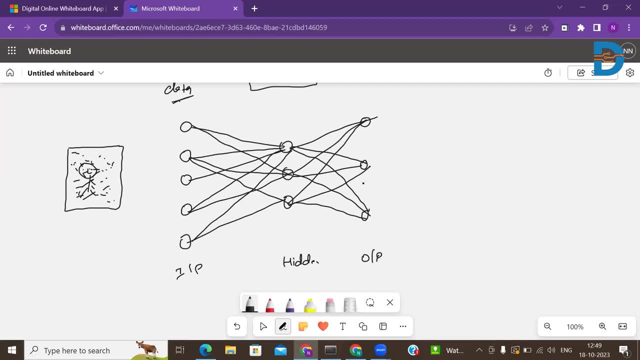 after having the noisy input, then the decoder machine takes the data and simply it gives me back with the no noise or noiseless input. So simply it takes this and you know when you do it it will be noiseless. When you do it you will find it out that you get a noiseless, complete, nice picture. 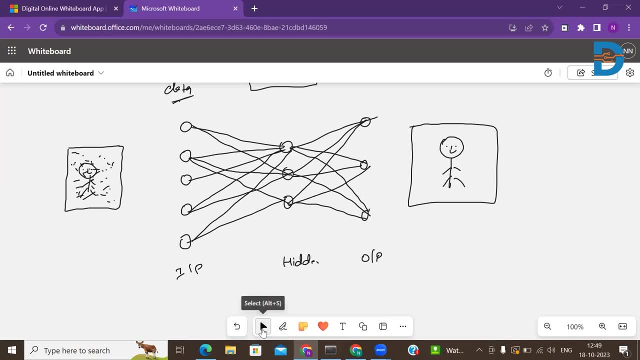 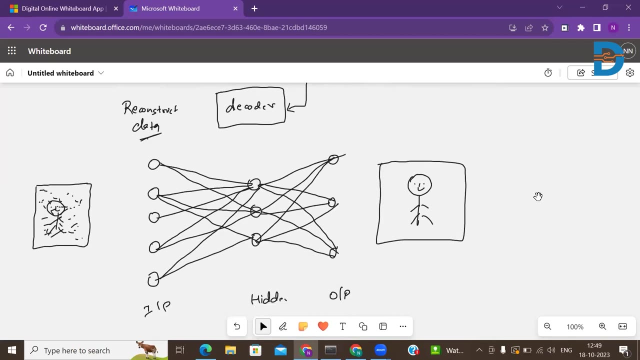 So, of course, that's one of the benefit of applications of autoencoder. Now, talking about the one of the more application of autoencoder, that is your feature learning. If you talk about the feature learning, well, feature learning is nothing. Feature learning is all about taking up. 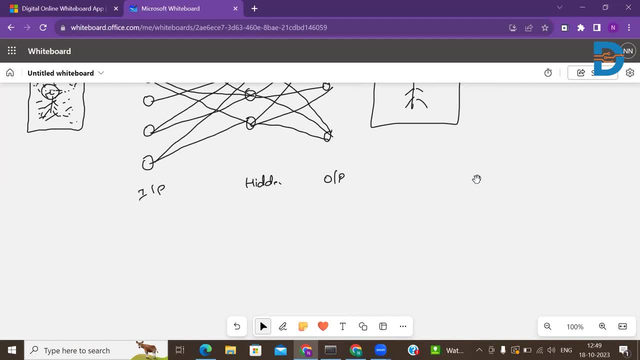 the data and, you know, converting it back into a lower dimension space. So autoencoders can be used as feature extractor for classification or regression task. Autoencoders, can, you know, take an unlabeled data to learn efficient coding about the structure and can be used for supervised learning tasks as